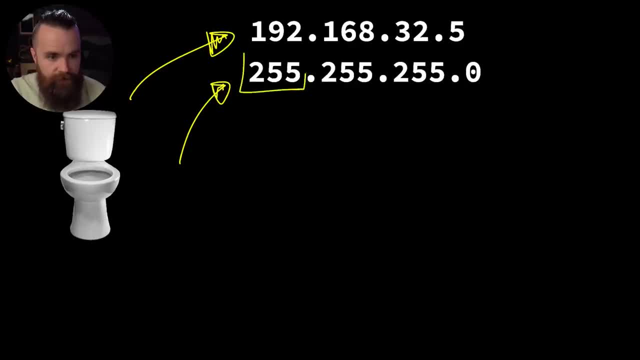 And you may even remember our little hack. Remember here: if we see a two, five, five in the subnet mask, we know that the corresponding octet or the corresponding number in our IP address is frozen. Just, it's done. It can't move, It won't change. 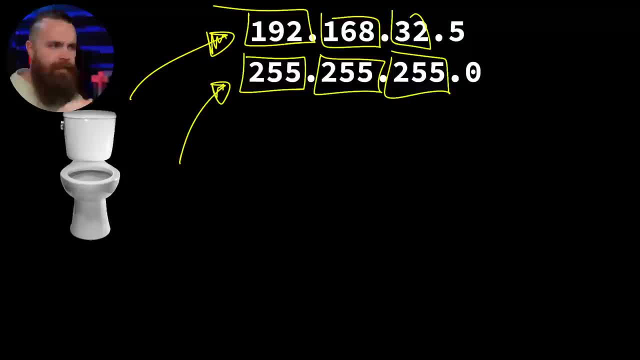 But the big question is why, Like why, does two five, five mean that number stays the same? What's actually happening here? What's the subnet mask doing? Why is it two, 55?? And this episode we're going to pop the hood on that. 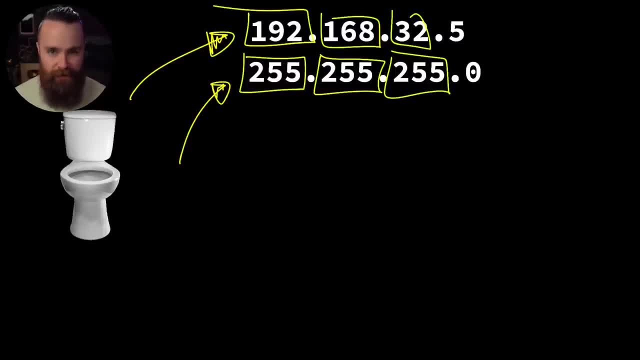 We're going to see what the heck is happening. Why is it doing what it does And why is the subnet mask so important? Now, in the previous episode, I gave you superpowers. You are now able to decode matrix computer code. I think, uh, yeah. 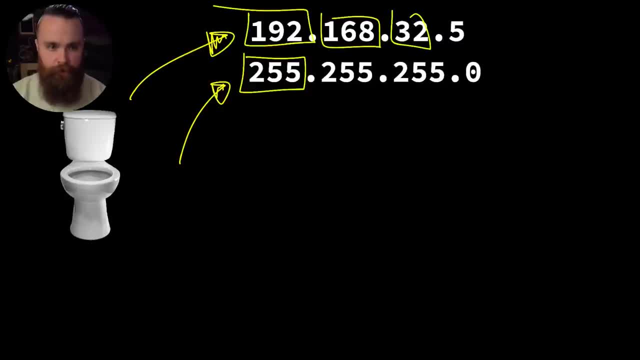 you can look at an IP address and convert it into binary, the language of computers, and you can convert it back And actually real quick. pause the video and see if you can convert our current IP address- the IP address of my toilet- and to binary, Keeping in mind, 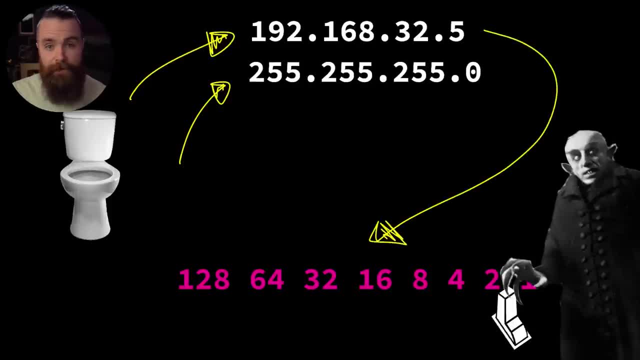 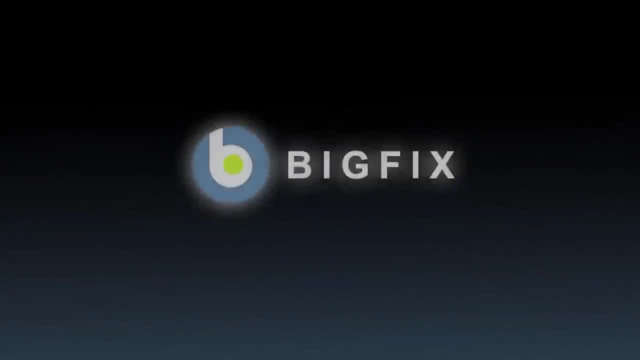 this will be a lot easier if you use the help of our handy Danny chart and nose for auto. So pause the video and go Hey time for a coffee break. And this coffee break, in the entire video, is sponsored by big fix. Oh, that's good. Now, while you're sipping that coffee, 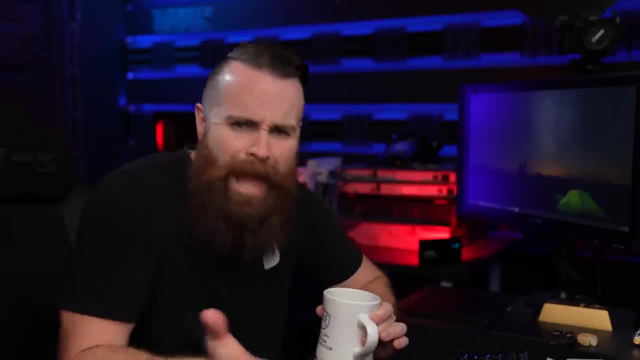 let's talk about something a bit scary. Cyber breaches you. you know they happen. They happen all the time: Solar winds, Equifax, Google, Octa, and then like log four J, that was crazy, Not to mention ransomware. 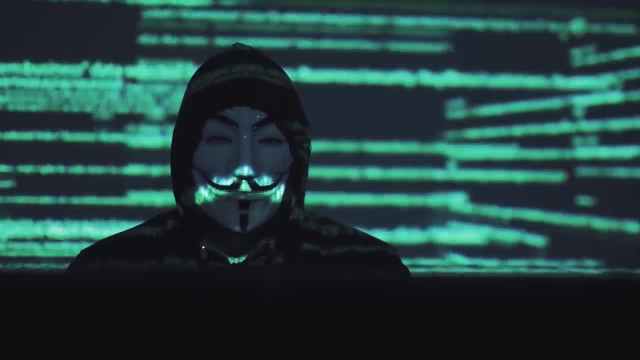 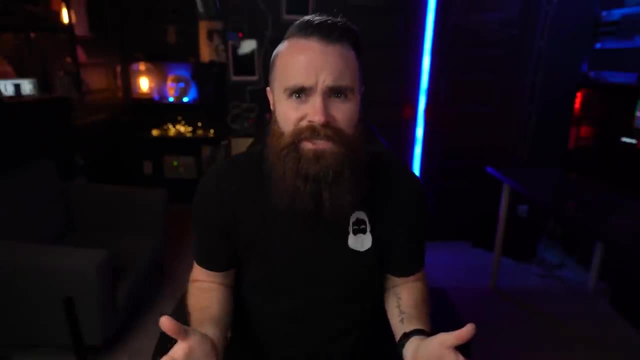 basically just lots of bad things happening to companies, making them lose money, making them lose your data on the dark web And, ultimately, they lose respect. Now you're probably thinking: why does this keep happening? Why haven't they stopped this? You know what? actually? I'm kind of surprised this doesn't happen more often, because here's the reality. managing it, infrastructure for large companies or even just small companies, is crazy hard. Actually it's kind of almost impossible. Hundreds, sometimes thousands, tens of thousands of end points that you have to make sure. 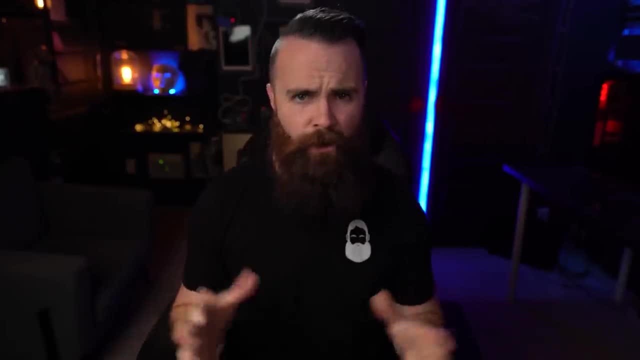 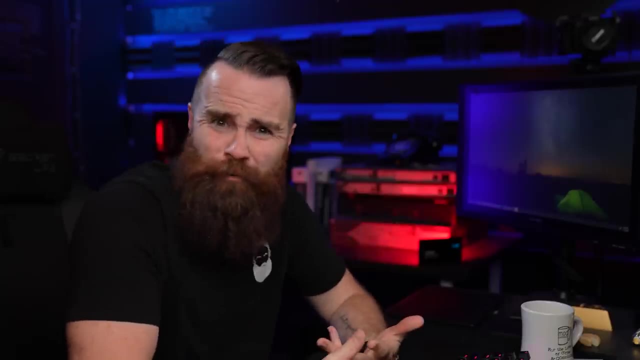 stay safe and adding to the complexity, They're not all the same right. They're not all in one place Like the office. they're gonna be at someone's house, you know, working from home, coffee shops and the cloud, And also they're kind of all different right. Like they're running different operating systems like iOS, windows, Linux, and it could be anything from a laptop to a phone to a kiosk And I know you probably have the situation cuz it's happened to me. You may have this old server that running this ancient 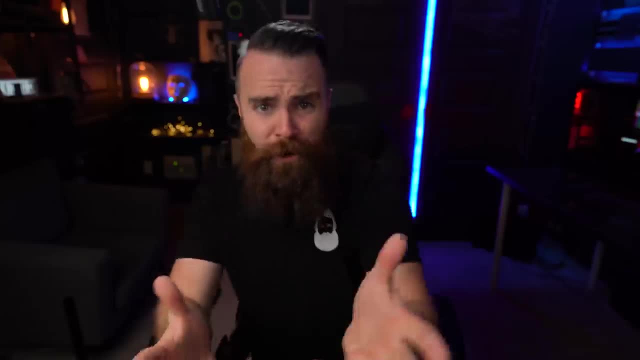 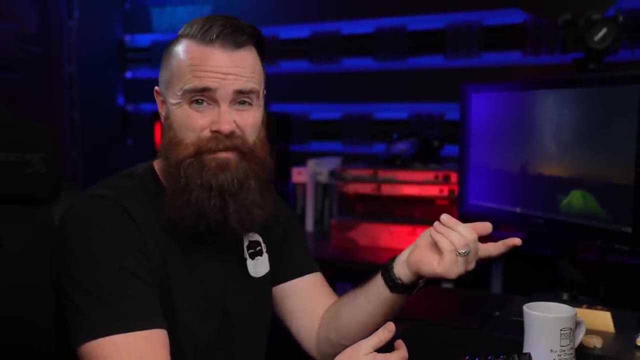 modern version of Linux, sitting underneath someone's desk in like Kansas or something. How are you going to find and update that when you don't even know it's there? And the reality is it only takes one of these devices to leave you vulnerable to a massive hack. So are you scared? yet One more sip of coffee. 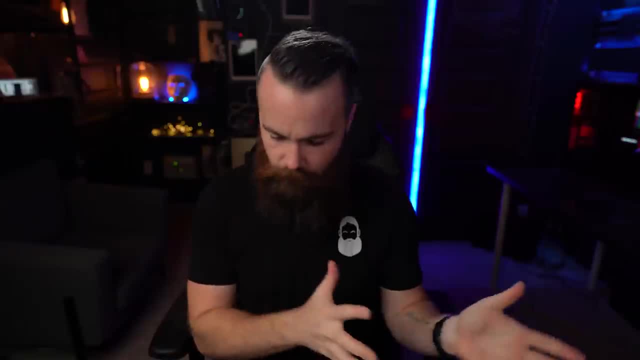 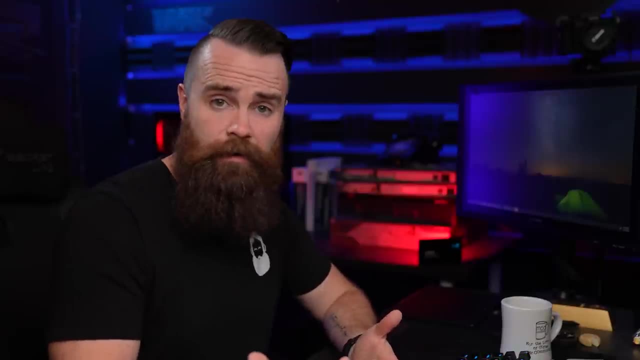 I told you it wasn't gonna be an easy coffee break. So how do companies, small to large, handle large it infrastructures of things that are everywhere all at once? Because some companies do handle it. Well, these are the companies you don't hear about because they're not getting hacked. 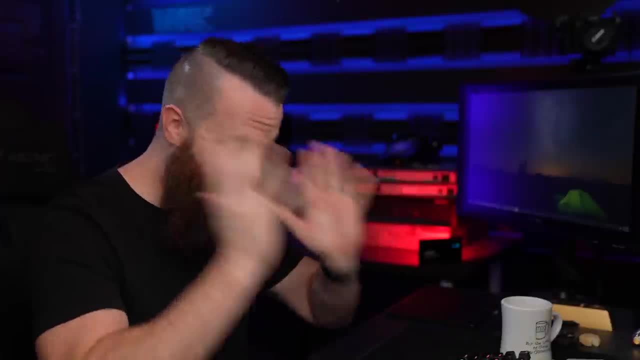 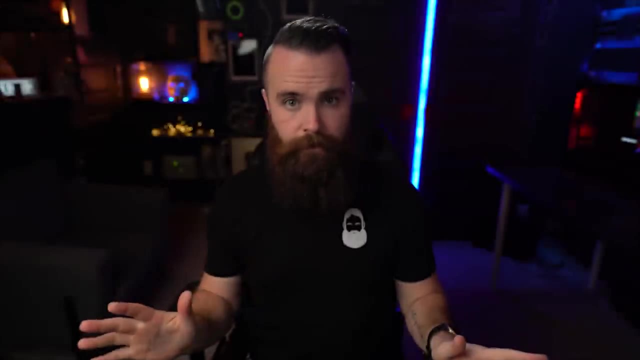 They will use solutions like HCL's big fix, which is Totally awesome, because here's what it does: It will automate the discovery, the management and remediation of all end points, And when I see all, I mean stinking all. 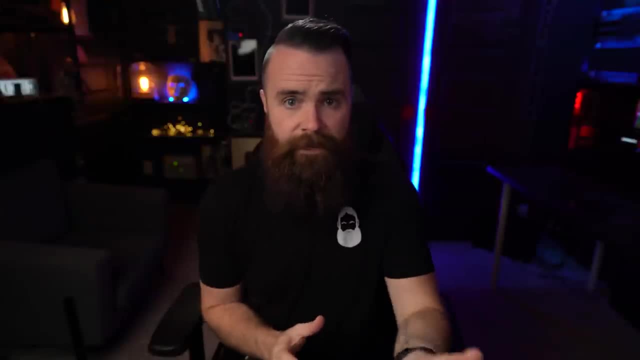 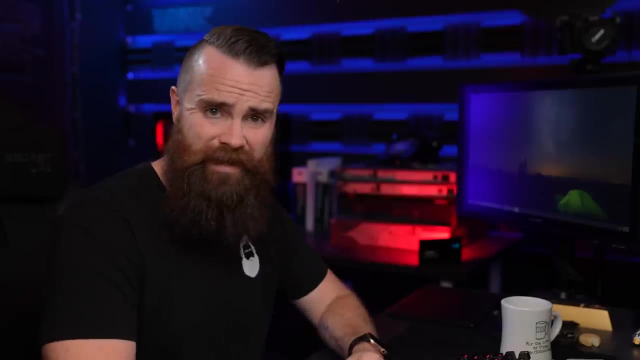 whether it's on-prem and your data center at someone's desk in the office, at their home office and then Antarctica, or under a desk in Kansas collecting dust. And it doesn't matter what OS they have: It could be Linux, Mac, iOS, whatever. 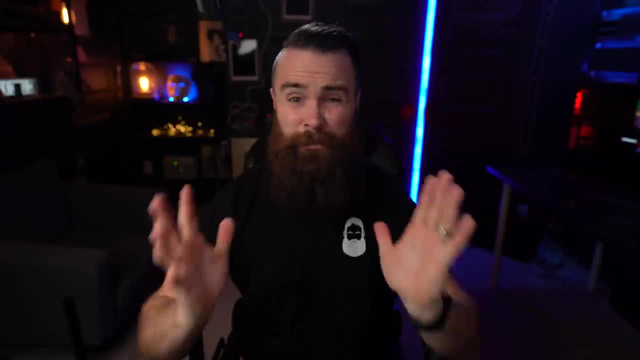 They can manage it, And you can do all of this from a centralized console. It teams can deploy patches and updates to their entire it landscape. Again, no matter where it's at, it could be sitting in someone's pocket, It could be. 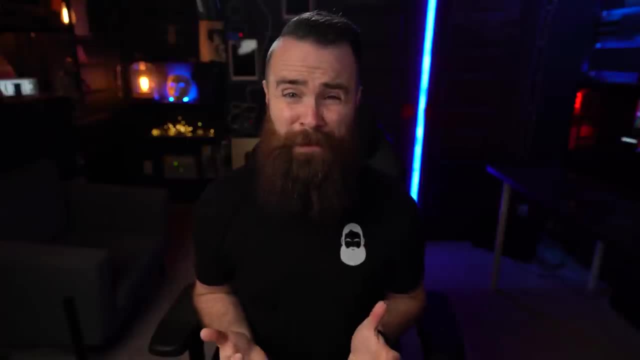 you know the phone or something, or the old grandpa. Now, I've been there, I know the pain. If you're an it operations or it security, how nice would it be to just be able to manage everything with one tool and also. 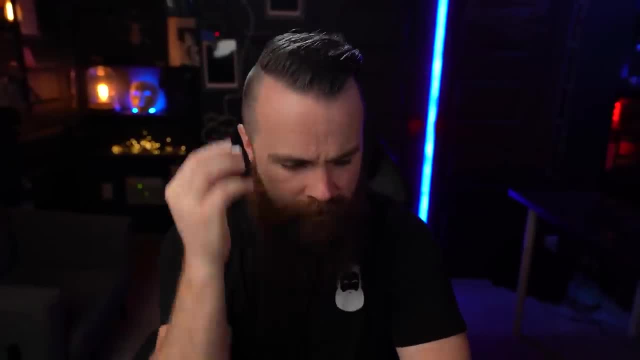 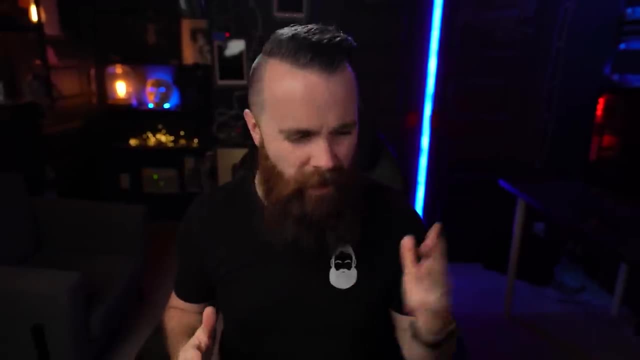 like just have a handle on things, know where everything is Cause I know, as an it admin and really just anyone in it, you're thinking you have that sneaking suspicion. Is there something I don't know about my missing? something that update that? server. a new vulnerability comes out and it's like the most disgusting one in the world. It's gonna bring down your company. You're like: I don't know if my stuff is updated. I don't even know how to find all the stuff. 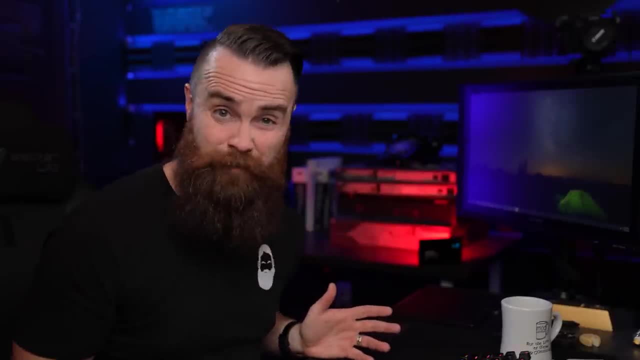 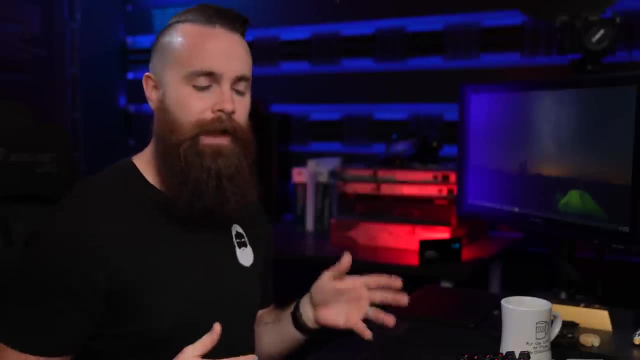 That's where tools like big fix come in. It'll give you better collaboration between teams, Cause- you know it- ops security. Everyone is gonna know through one console where things are. what's going on? Is this server patch? What OS is this running? 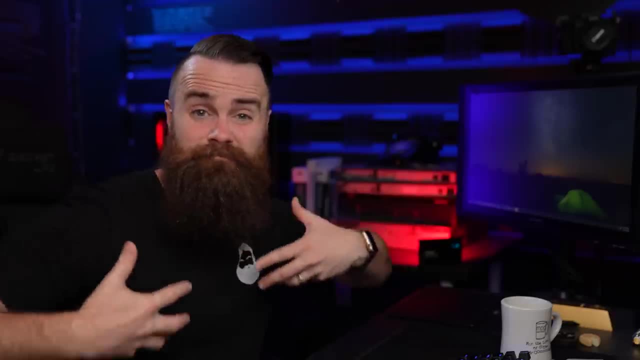 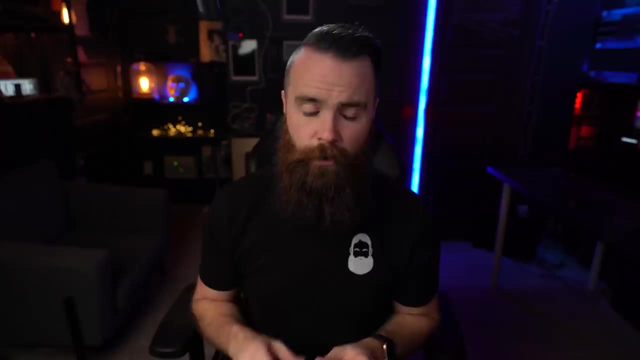 So you'll be able to cut down on operational costs and you can enforce what's called continuous compliance, which again when audit time comes around. So I know like when I say audit, you get chills, and I've been through a few and they, they're terrible. 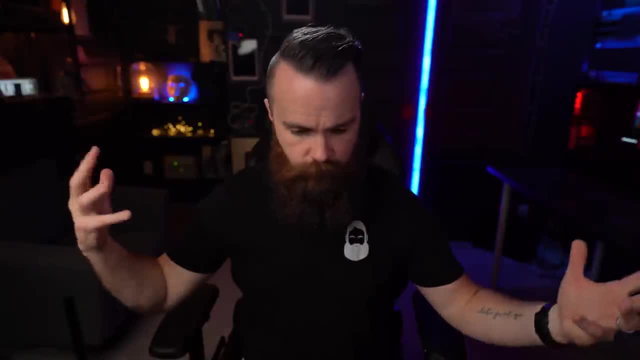 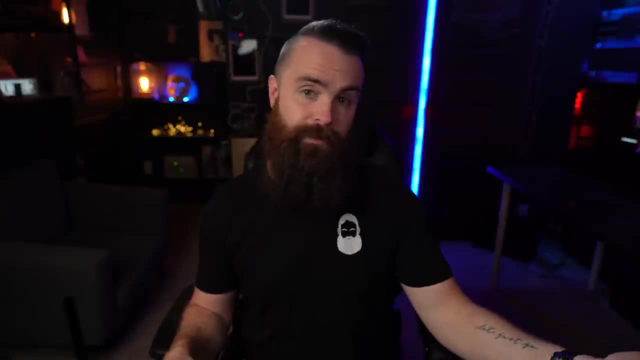 but with big fix you've got your arms around everything. They generate these Amazing reports automatically for these compliance standards, saying Hey, yeah, everything's up to date. or Hey, we know the system isn't patched. We're gonna patch it real quick with one button. And a lot of these fixes are automatic. They use intelligent automation. They even have these things called fixlets, which sound like chicklets, which provide all these benefits and make it really easy to just deploy fixes to things. And because it'll automate a lot of the tasks you might like be doing. 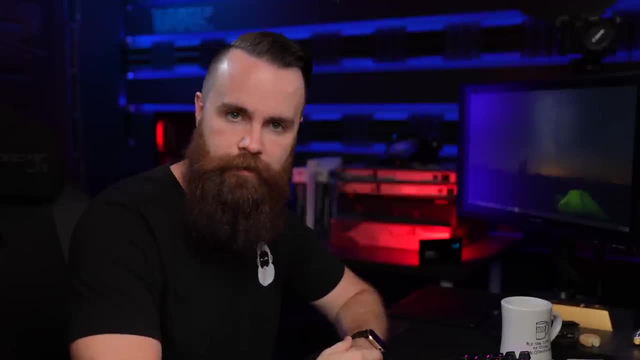 manually right now. like what are you doing today? You're probably just gonna be packing servers right All day. Do you have to pull up a report? I mean it's just a pain, right, But big fix will free up that time. 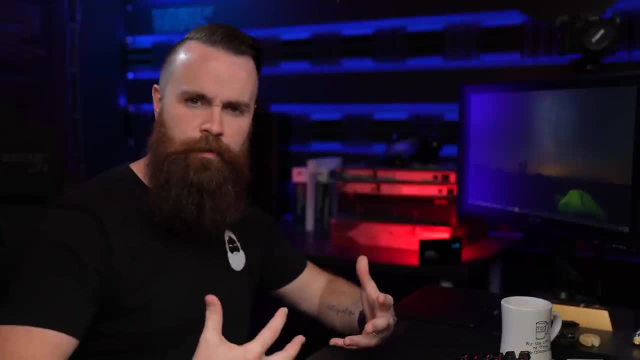 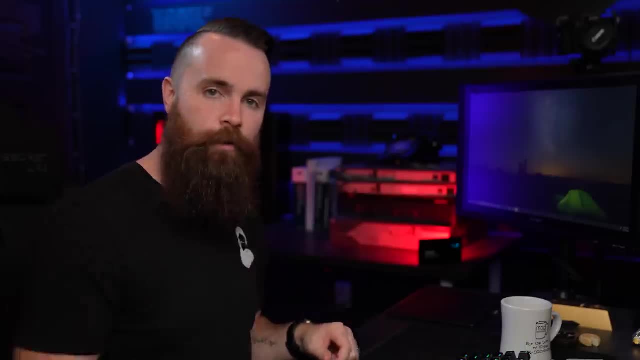 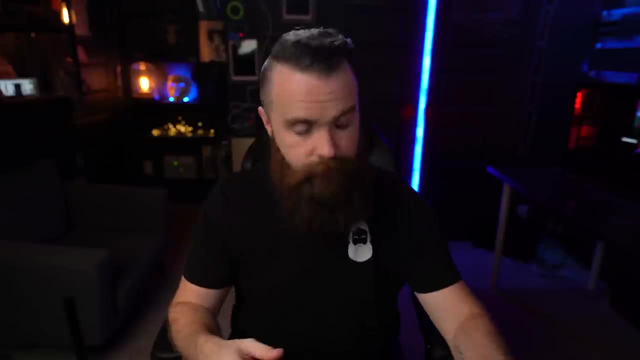 lower that anxiety and stress. check out big fix. I got a link below big fixcom. You can actually sign up for some free training to see, Hey, what can this do for me? That can do a whole lot. And Hey, thanks for having some coffee with me. Let's get back to the video. 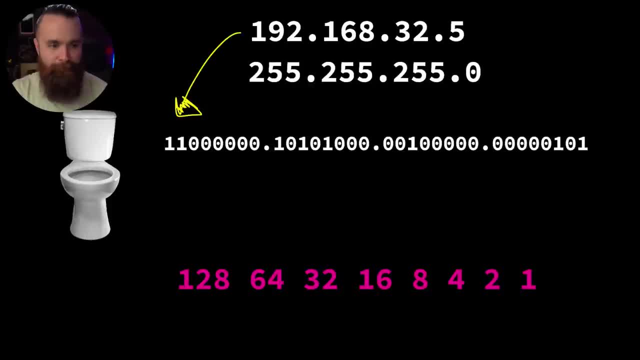 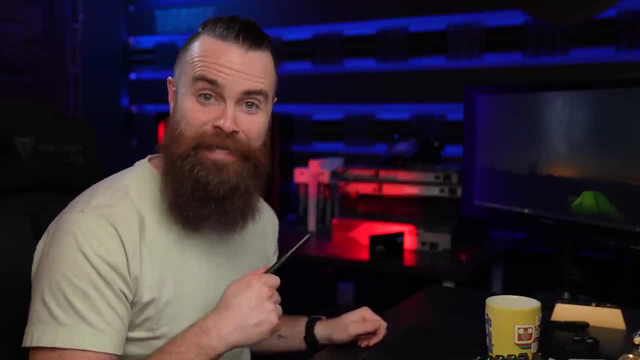 Unpause, coffee break and done. This is my toilets IP address and binary and computer code and matrix code. And if you're wondering how did he do that, Go back and watch the previous episode. I'll show you how. it's remarkably simple and kind of fun, Actually No. 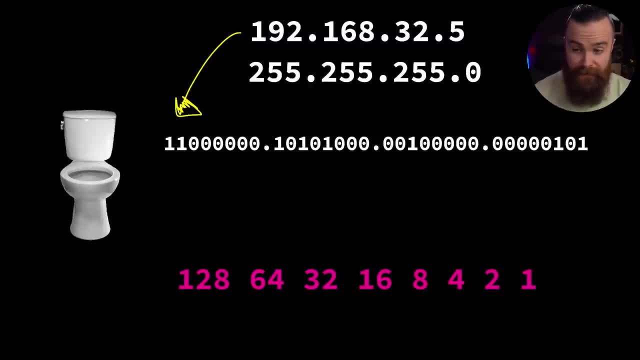 it's very fun. Just go do it. Now. what we did not do in the last video is convert our subnet mask into binary, which is something we totally can do, should do and will do right now, And this one's kind of remarkably easy. So, for example, 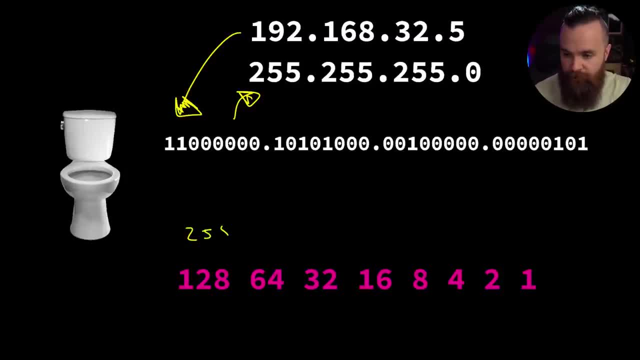 if I'd bring my first number down here, my first octet, 255, and I wanna see if the first bit is gonna be on or off, one or zero? can 128 be subtracted from 255.? Uh, yes, a hundred percent. Yes, it can. That first bit is on. 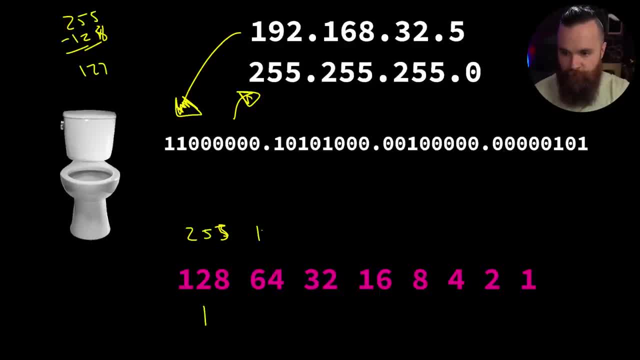 So 255 minus 1 28 gives us 1 27.. Bring that over here. Can we take 64 away from 1 27?? Yes, we can. That bit is on. 1 27 minus 64. Gives us 63.. Can we take 32 away from 63?? Yes, we can, That bit is on. 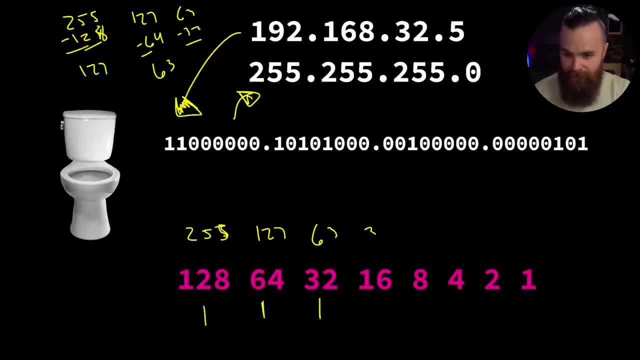 So 63 minus 32 gives us 31.. Now I'm gonna give you a little spoiler alert. We'll be able to turn every bit on. That's the secret. We will go down every single digit until finally that 2, 55 is zero. 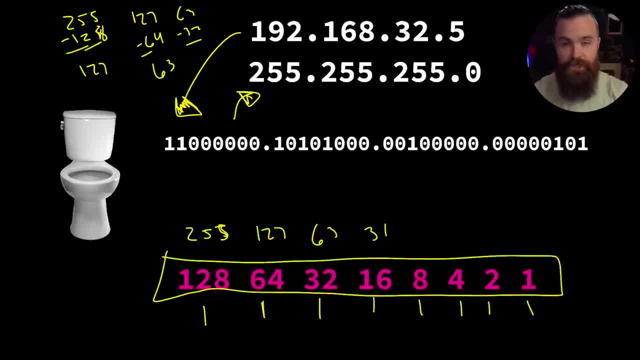 because if you add all of these numbers together here in our chart, you're gonna get 255.. Go ahead and do it real quick. Let's do it with our calculator: 1, 28 plus 64,, 32,, 16,, 8,, 4,, 2, 1,. 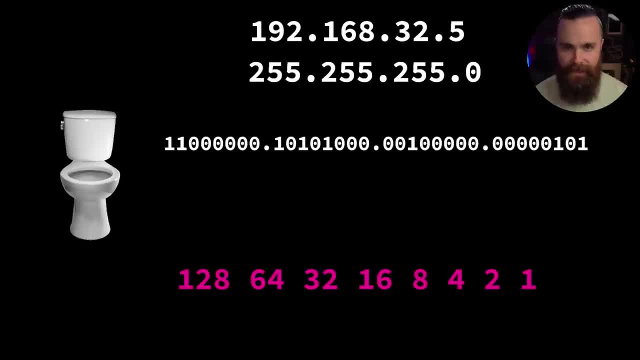 255, knowing that 2, 55 means every bit and that octet will be on. go ahead and finish out the mask. It's kind of easy right? This is our subnet mask converted into binary, all ones all the way across in the first three octets. The last one, also easy, because zero and binary is. 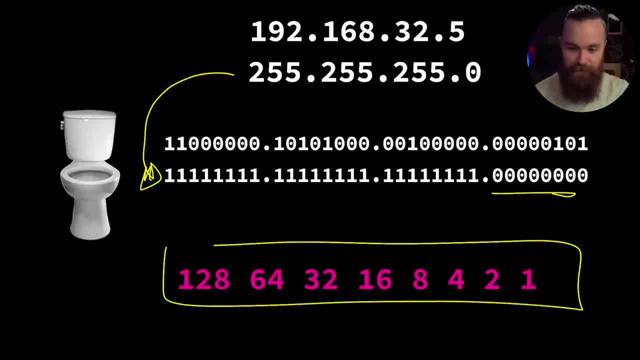 still zero. All the bits are off Because you can't take any of these numbers away from zero. Now here, here is where it's all gonna come together and make sense, and and and why we're converting stuff into binary. Anyway, like, what's the point? 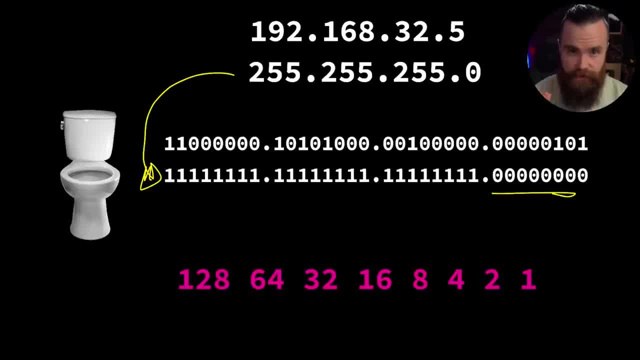 Here's the point, Because if you listen closely, these ones and zeros in our subnet mask, they're speaking to us, They're telling us something, They're whispering things about our network dark mysteries. If you can't hear, I'll go. I'll go ahead and tell you, sorry. 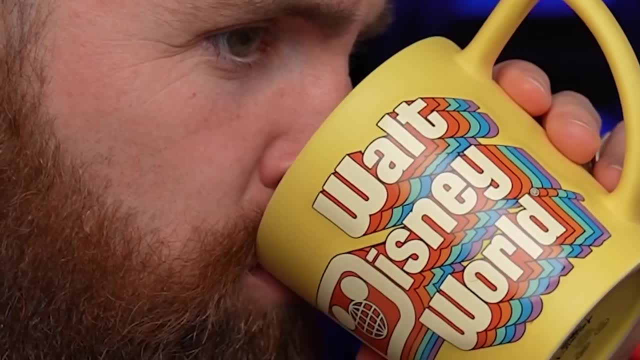 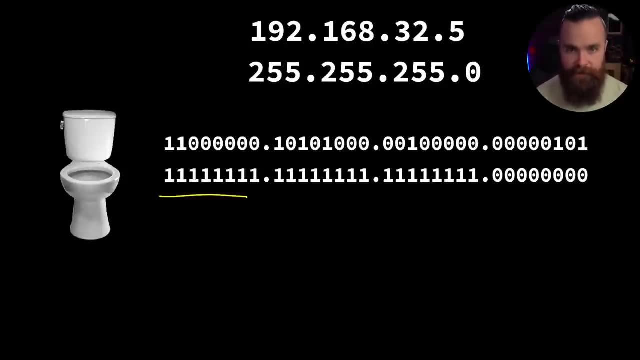 That was stupid. but stick with me. Take a sip of coffee. get excited When you're looking at the subnet mask. tell us. they whisper to us which part of the IP address are the network bits. So looking here we can tell that, dude, we got lots of ones. 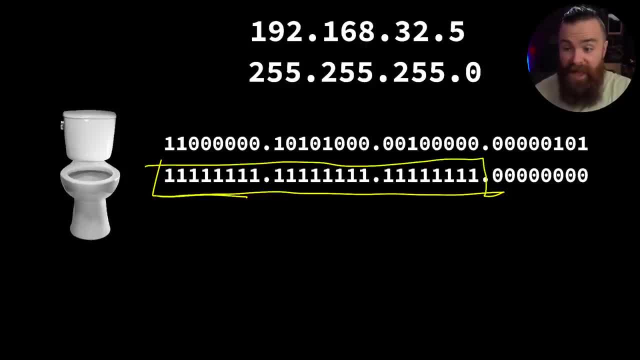 all ones all the way down in our first three octets, which means every one of these bits appear in our subnet mask. all the way down through all three octets are the network bits. So network bits, AKA the part of the IP address that won't change and tells us which network 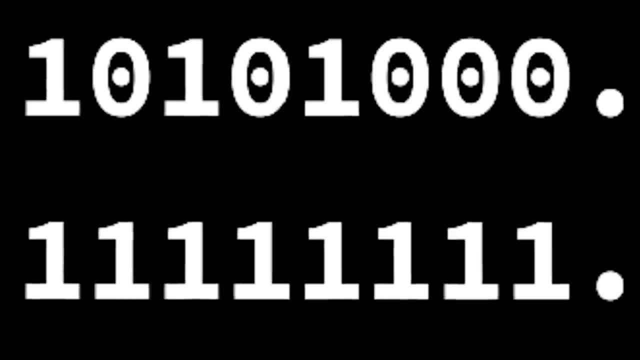 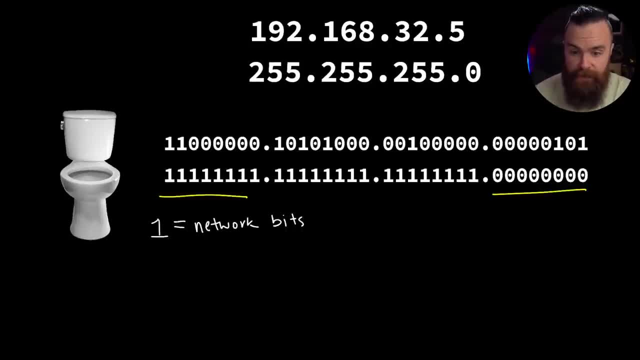 we're on And then it's also whispering something else to us here. Listen closely, Listen the zeros. they tell us which parts of the IP Address our host bits. So looking at our mask, we can see that the entire fourth octet is all zeros. 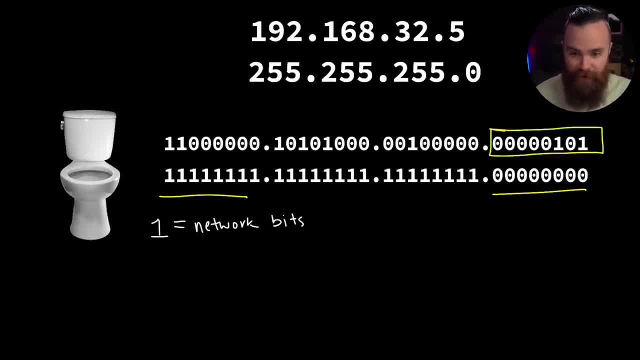 So we know in the IP address every bit and the fourth octet will be a host bit, Meaning each of these bits can be used to create an IP address and that network and be assigned to that host. Now I know this is weird. 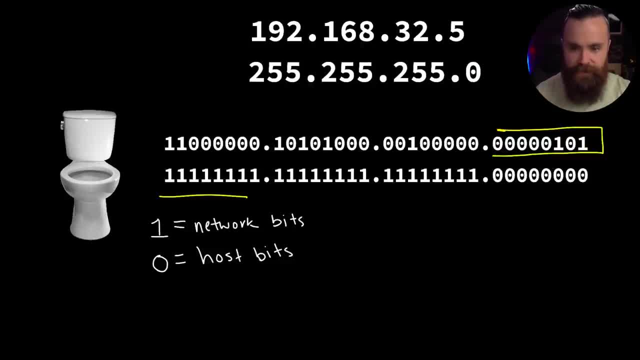 but here's one example of how this is cool. So the zeros tell us which bits are host bits, which also tells us how many possible hosts there are in the network. All we gotta do is count the number of bits. So, looking here at our subnet mask. 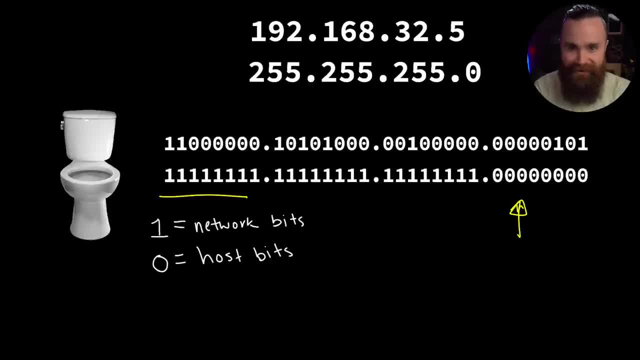 how many bits are zeros? I mean, they're all in the last octet. They're eight, eight zeros. And I know you're probably thinking: well, Chuck, I counted eight zeros, but I know I know, looking at this network. 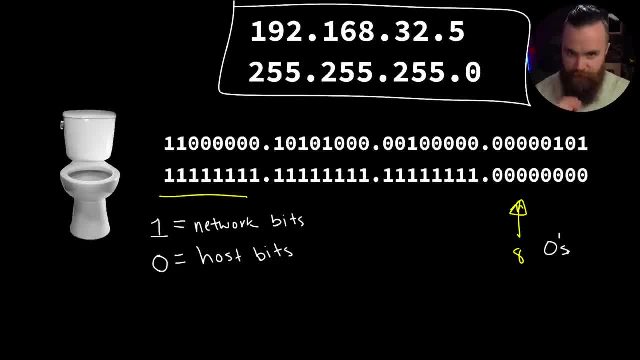 this network can have more than eight IP addresses. and you're right, We're not done yet, because there is a formula with this to see how many hosts can be in any network. Here it is. This is so powerful. Just put this in your pocket, man. It's gonna be two to the power of zeros. 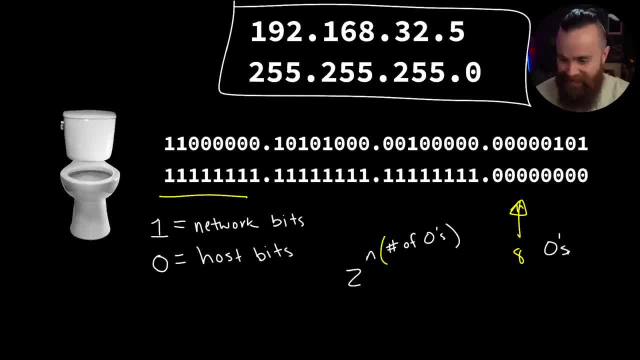 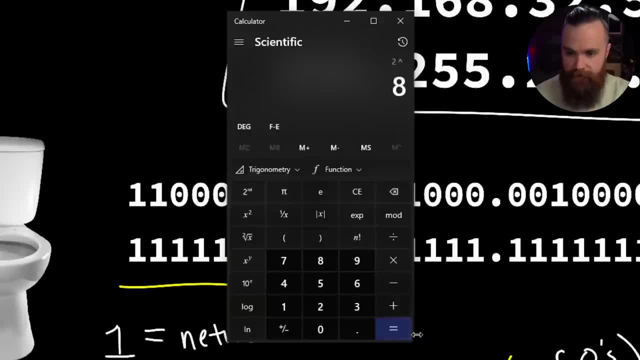 How many zeros there are. So, for example, our example here: let's grab a calculator. If I take two- and I do my little power two of something, the carrot right, two to the power of how many zeros, eight, that gives us 256, which is absolutely correct In this network. 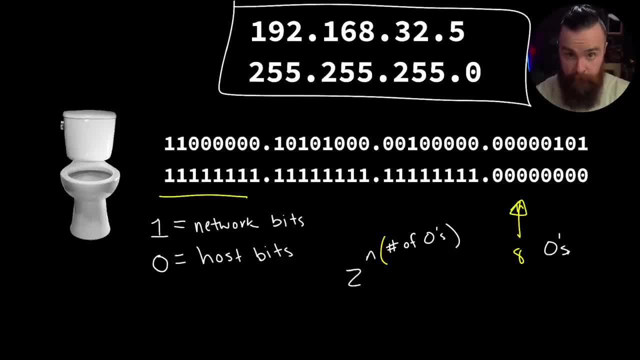 we can have 256 IP addresses. Now of course we can't use all of them. We have to subtract two to account for the subnet ID or the subnet address, and the broadcast address, the first and last IP address in the network, which gives us a total of the 254 usable IP addresses. 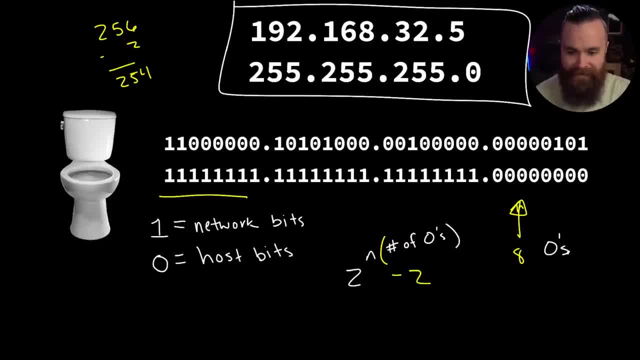 So the official formula would be two to the power of number, zeros minus two, because every network will have those two IP addresses reserved. So what this unlocks is something crazy Powerful, because we know, if we count the zeros it gives us 254 usable IP addresses. But if we're like Hey, 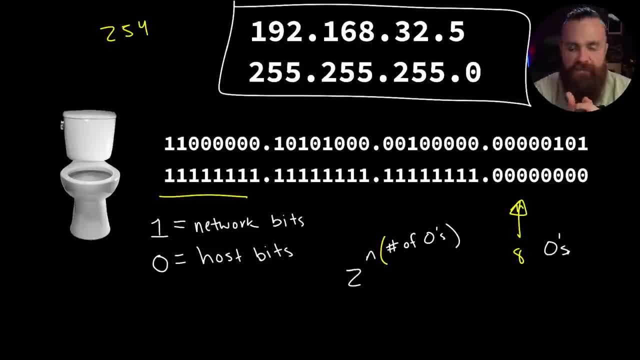 I need more than that. My network I need. I need like 500 IP addresses in that in my network. How do I get more? The simple answer is we need more zeros, We need more host bits to have more hosts And to do that, 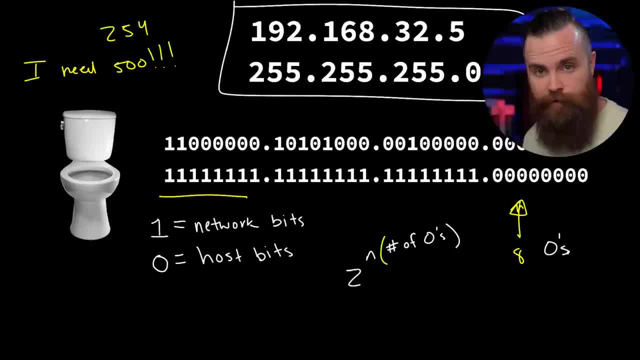 we're gonna borrow or we're gonna steal from the network. We're kind of like peeking behind the curtain of the next video or we're really gonna break it down. I just wanna give you a peek. I can't tell you too much. 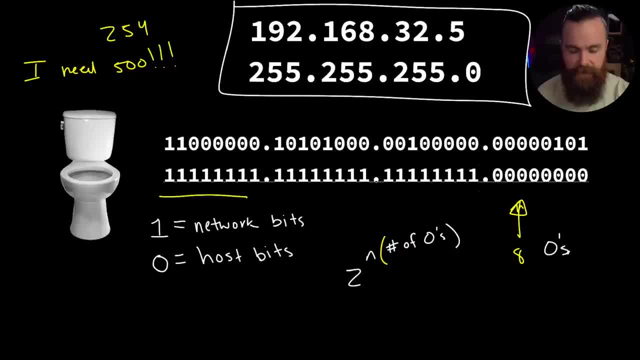 But if I come over to this subnet mask here, I'm gonna take away one of the networks bits. I'm gonna take this last one and convert it to a zero. You're on the host team, Welcome. So now, with that extra zero, how many hosts can this network have? 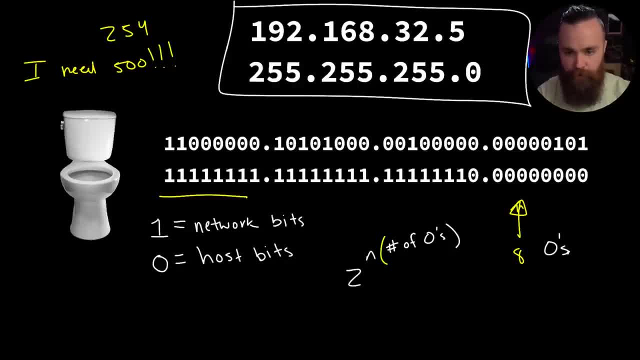 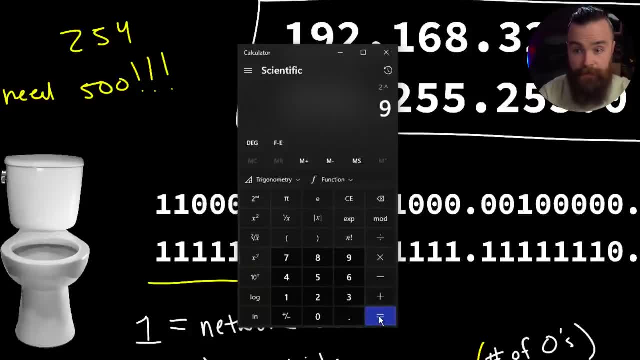 Let's try it out. Let's use our formula two to the power of number of zeros. Well, now we have not eight zeros, but nine zeros. So with our handy dandy calculator, two to the power of nine will give us 512 addresses. 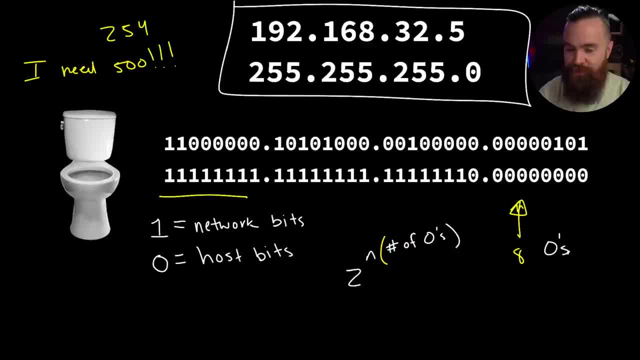 which, minus two, gives us 510 usable addresses. So right here, I want you to understand what just happened. We converted our subnet mask and our IP address into binary. Well, for this moment, that was just like a, a, a thing you had to learn to do an. 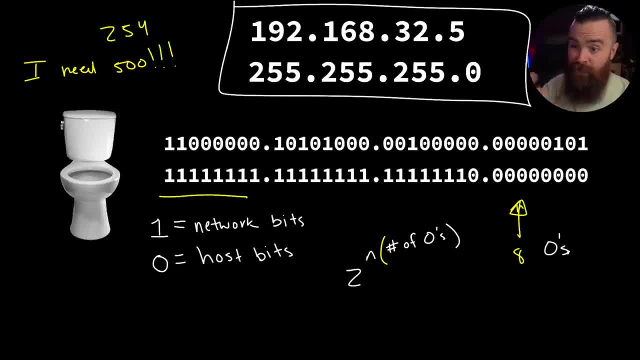 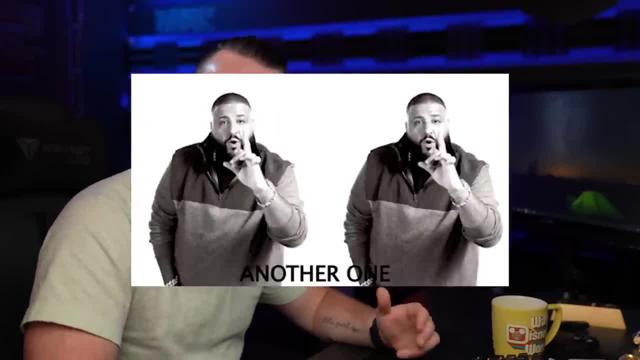 exercise. Now it's coming together, cuz what we just did is we went from having 254 available host And we said no, not good enough for me. I want more IP addresses in my network, Another one, another one, I want more. 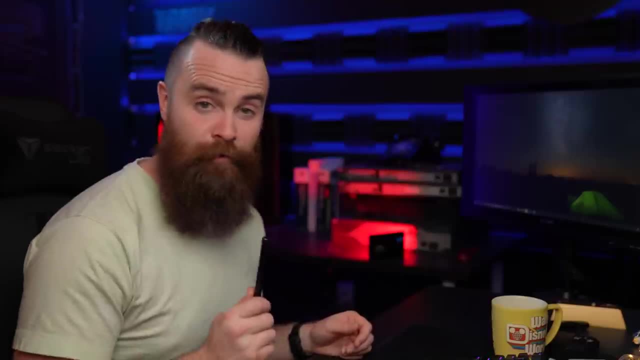 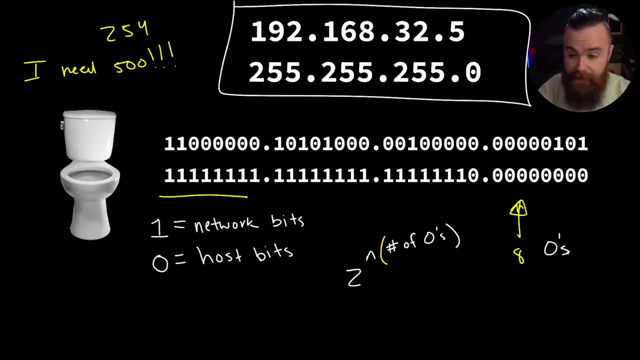 I want 500. So we stole a bit from the network side, giving us more host. that that's subnetting We. you just subnet it, Because all really subnetting is is changing The subnet mask to suit our needs. So here's a challenge for you real quick. 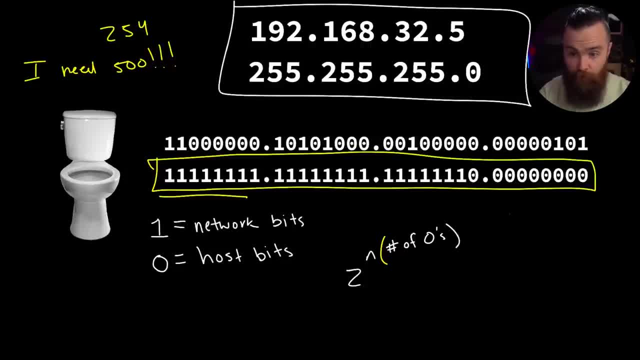 We changed our subnet mask, which means the value in decimal is gonna be different. It will no longer be two five five, two five, five, two five five zero, Because we changed something. We changed the third octet. So real quick. 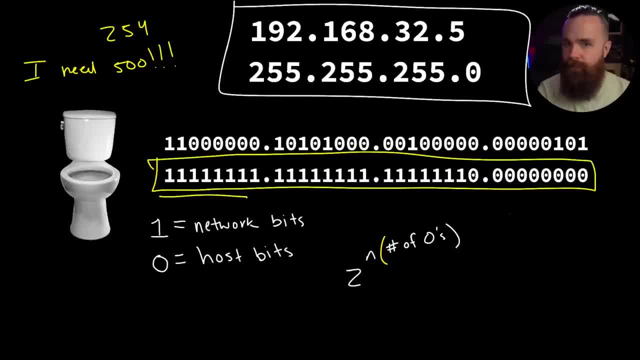 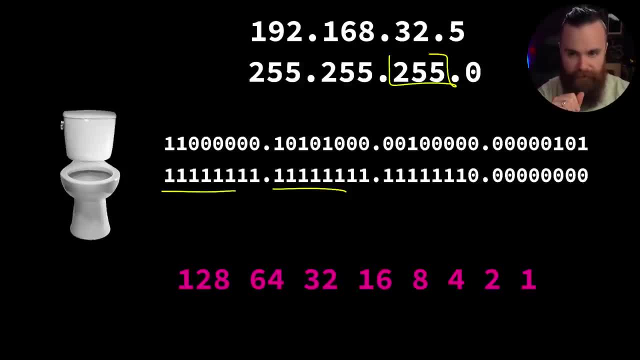 let's convert it back to decimal, back to the regular version of it, and see what it looks like. Now, right off the bat, we know that the first two octets will be the exact same- They're all ones- but the third one it won't be two 55 anymore, It's gonna be different. 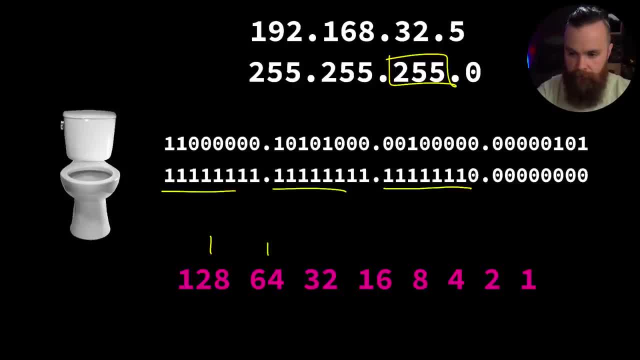 We know the first. let's see: seven bits here are gonna be on: bam bam, bam, bam bam bam, just like that, And all we're simply gonna do is add these numbers together and our result will be- and you may have been able to do this in your head- The result will be two, 54.. 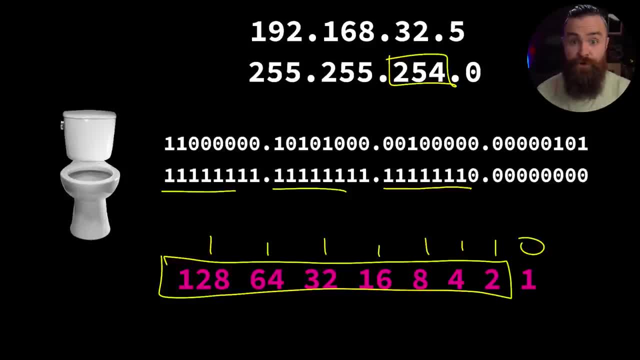 That's our new subnet mask with 512 possible IP addresses, or 510 usable IP addresses. Now, what just happened here was nothing short of magic, And I'm leaving a lot of questions unanswered, Like: Hey dude, what's our range of IP addresses? Like how, what's the network look like from like? 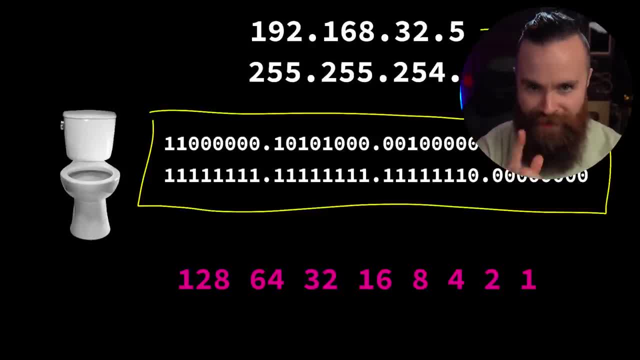 what IP address to what IP address. I'm not gonna cover that right now. We're gonna cover that in the next episode, where we're gonna break down subnetting and do a lot more of it. That's, that's what I'm trying to say. 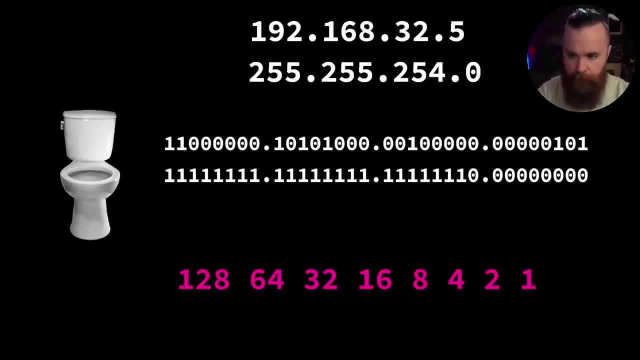 But one more thing before we end this episode I want you to notice: in our subnet mask the numbers are contiguous, which is a weird word I always love saying, cause it feels like continuous when I'm adding a G: contiguous meaning that the ones will always be in a row, Like you won't suddenly have one. 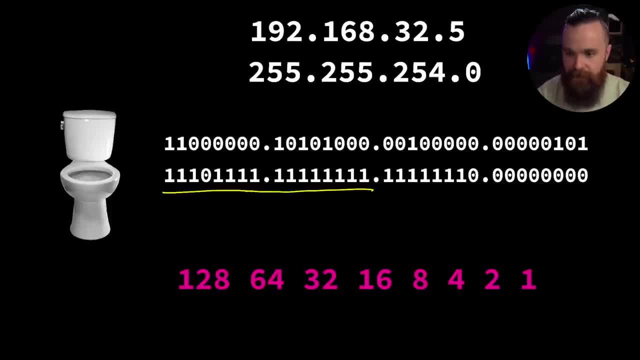 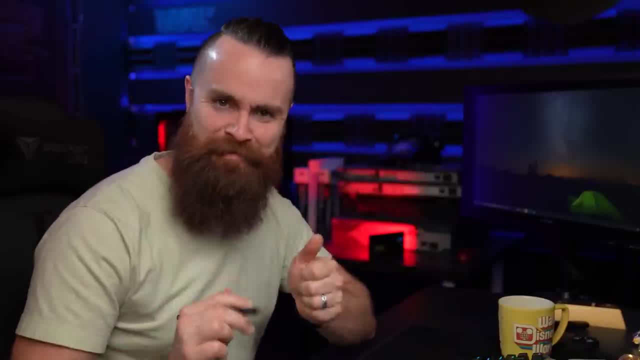 one one, one zero. No, no, that will never happen. The numbers are contiguous. It'll always be a row of ones and always be a row of zeros. So in this episode we uncovered a few of the deep, dark secrets of the subnet mask. 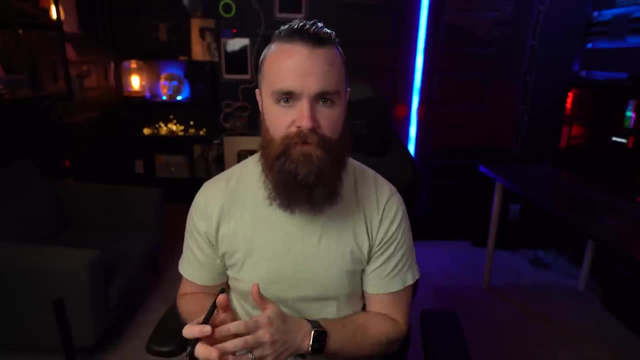 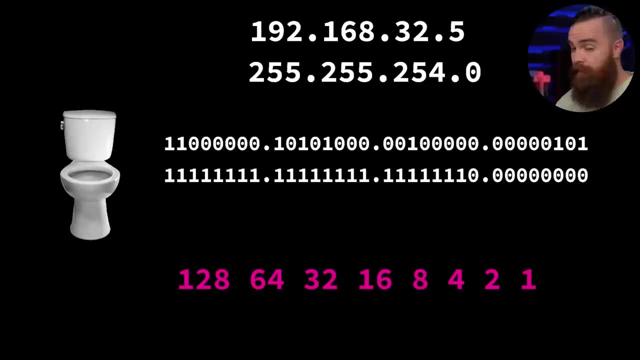 He tells us how big our network is, He tells us how many IP addresses we have. But in this episode we actually dove deeper into how that works and what's actually happening. And in the next episode we're gonna dive even deeper, because these ones and zeros. 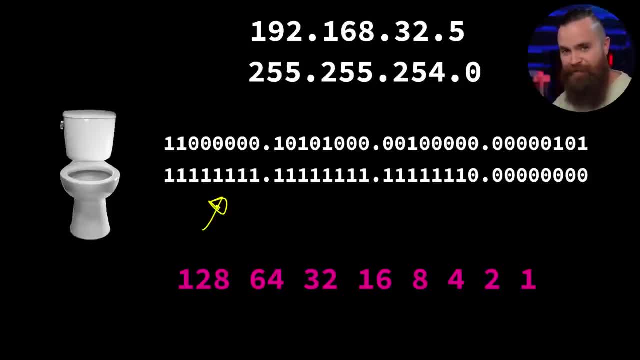 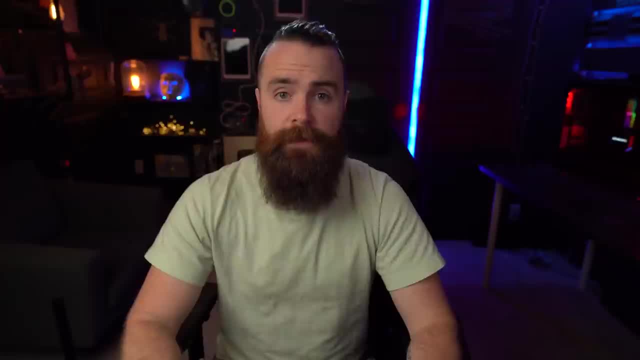 they're not done whispering to us. They have some more secrets that we haven't uncovered yet. So I'll see you then. And, by the way, if you want some extra practice converting your subnet masks into decimal and back to binary and vice versa, check out network Chuck Academy link below. 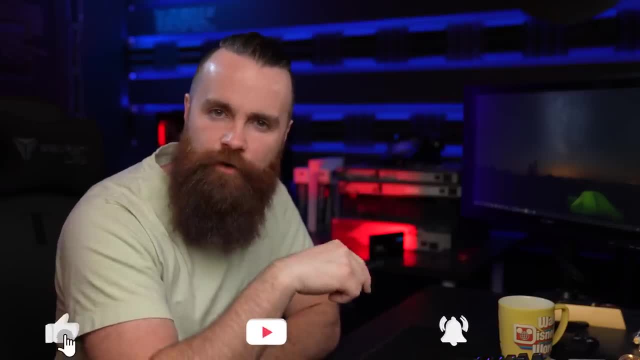 I've got a ton of extra practice for you. Oh and also, Hey, have you hacked the YouTube algorithm today? Let's make sure you do. Hit that like button, notification, bell, comment, subscribe. You gotta hack YouTube today, Ethically, of course. Yeah, that's all I got. I'll catch you guys next time.